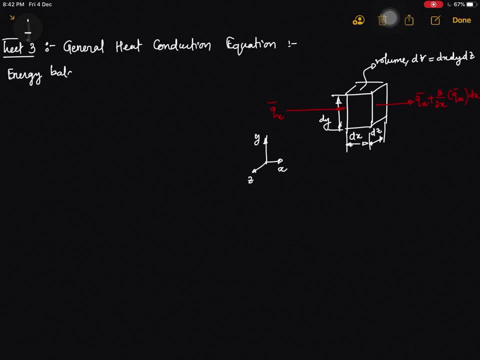 this equation is nothing but energy balance. So let's write the energy balance equation. So let's write the energy balance equation. energy balance, net rate of heat transfer plus net rate of heat generation within the body will be equal to rate of change of internal energy of the body or within the body. so this is the energy. 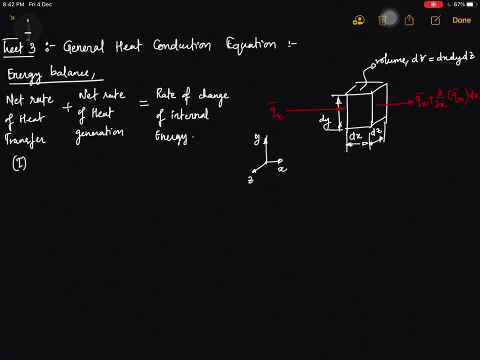 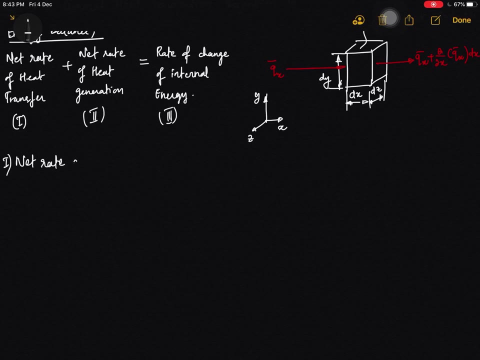 balance equations. so let's discuss each and every term. in this situations, this is having three terms, and this is first, and this is second, and this is the third term. so let's discuss each and every term. so let's first go through the first term, which is the net rate of heat generation. net rate of 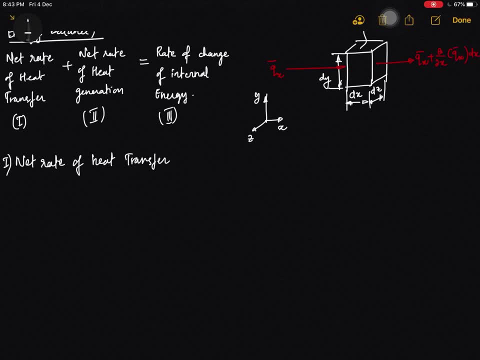 sorry- net rate of heat transfer through this particular element. so in this we can see that along x direction a heat flux qx bar is entering, which is positive, and this qx bar into dy, into which will give the area, and two other, it will give the rate of heat transfer, and minus q x bar, plus dou by dou x of qx bar into dx. 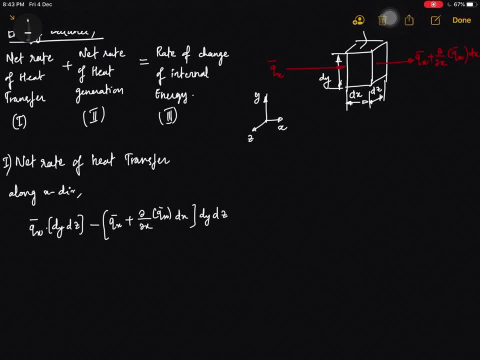 which is a heat flux that is leaving this particular element into dy, into dz, which is the area through this this heat flux is occurring, which will be giving minus dou by dou, so qx bar into dx, dy, dz. this is the area through this heat flux is occurring which will be giving minus dou by dou x of qx bar into dx, dy, dz. 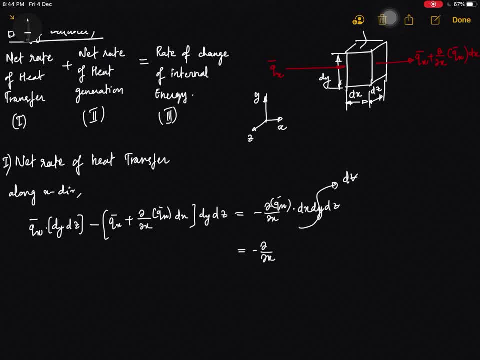 and this ds, dy, dz is nothing but the dv, so we can write this as minus dou by dou x of qx bar into dv. so let's note this element as qx bar is the heat flux through the x phase and this is the area through which the heat flux is occurring and together or the multiplication. 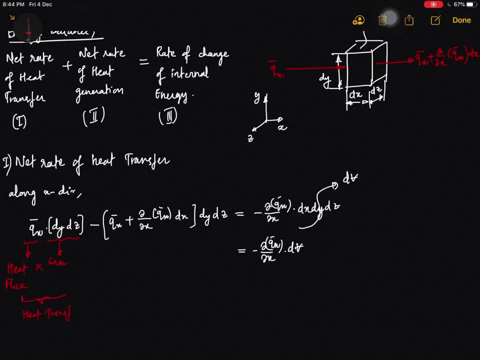 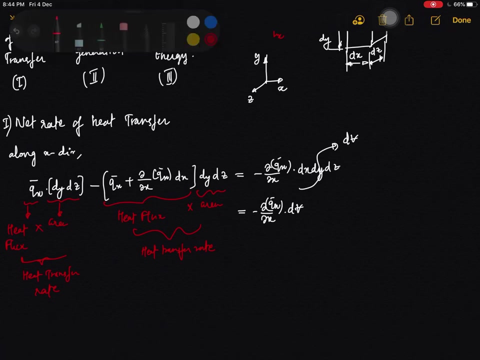 of this will give what heat transfer rate, heat transfer rate similarly, and this will be the heat flux and this will be the area, and together we will be getting heat transfer rate. okay, so this is the case in the long ds direction. so let's, let's, let's. 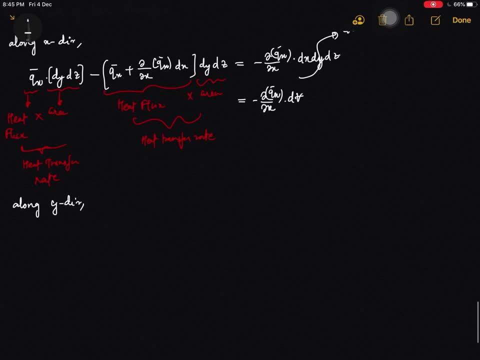 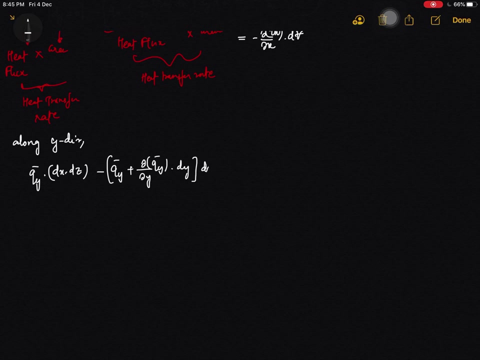 discuss similarly the case along the y direction. along y direction we can write qy bar into the qy bar is the heat flux along the y direction and this area will be dx into dz, minus qy bar, plus dou by dou y of qy bar into dy, into area will be dx into dz and this 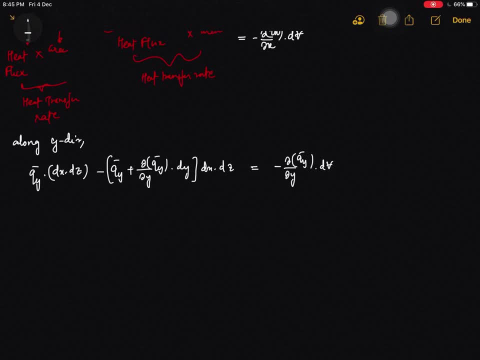 will be equal to minus dou by dou y of qy bar into dv. dx into dy, into dz is nothing but dv differential element. similarly, along the z direction we can write qz bar into area which is dx into dy minus qz bar plus dou by dou y is a dou of qz bar into dz, into the area. 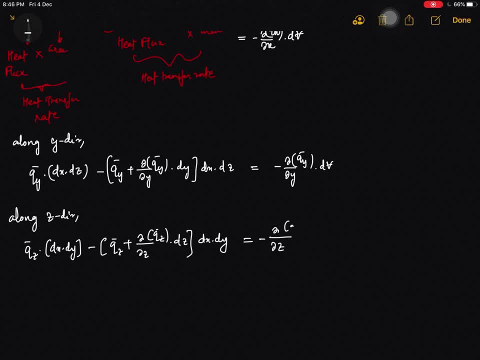 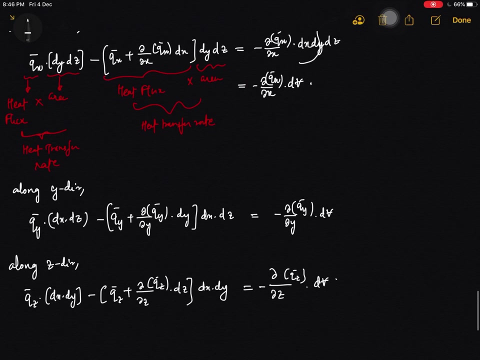 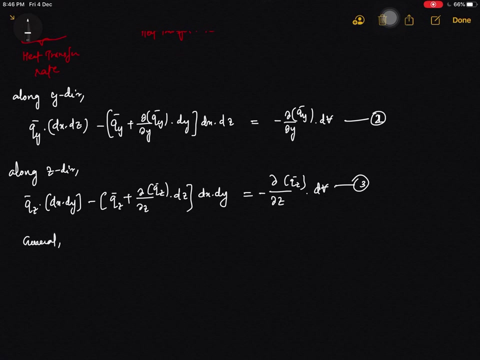 which is dx into dy will be equal to minus dou by dou z of q. z bar into this is dou, this is dou into dv. so these are the right transfer along x, along y and along z directions. so, comparing all this, we can write in general. in general, that is the heat flux or the heat. 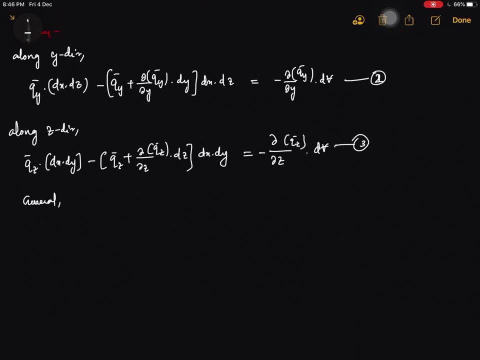 transfer rate that is occurring within the body along x, y and z direction. we can write it as minus along x direction, which is the unit weight of right cap, dou by dou x of q, x bar plus j cap into dou by dou y of q, y bar. 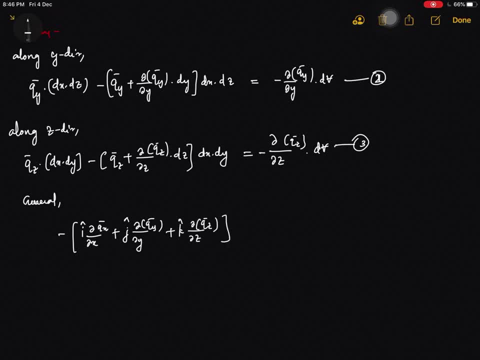 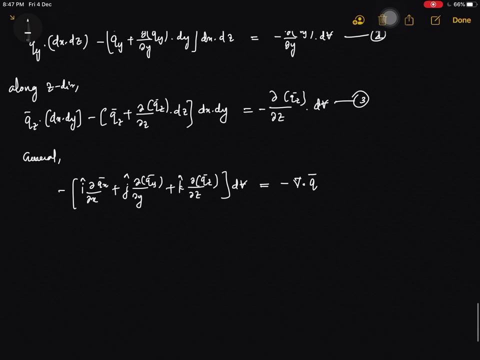 plus k cap of dou by dou z of q z bar into dv, so this can be written as minus del dot q bar and this q bar, which will be equal to minus del dot k, delta t. okay, this is explained in the last lecture, so please go through it for any. 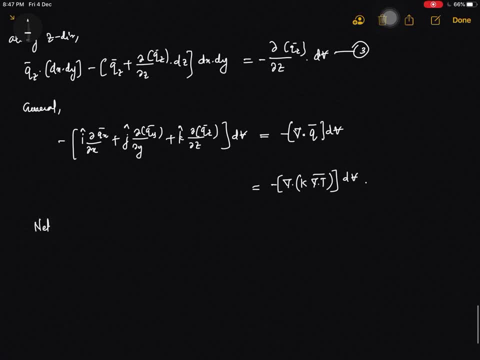 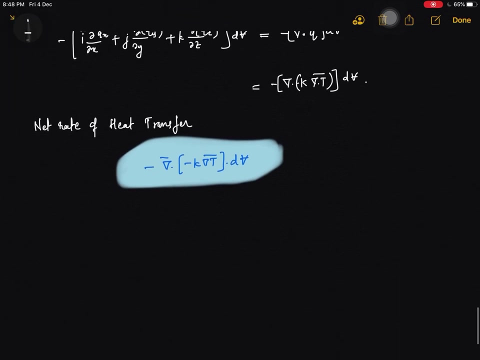 clarification. so in general, the net rate of heat transfer will be equal to: in general, net rate of heat transfer within the element will be equal to: we can write minus del dot, minus k, delta t into dv. okay, so this is the net rate through the element. there is a minus n over here, so 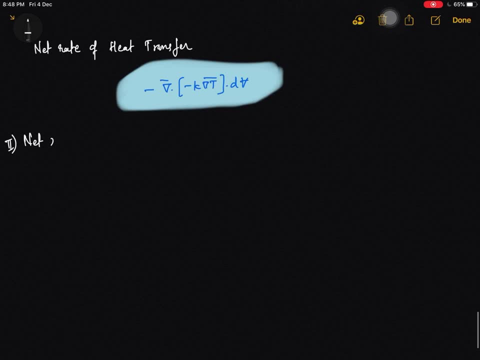 next let's discuss the second term, which is nothing but the net rate of heat transfer, which is nothing but the net rate of heat transfer, heat generation. so let's suppose qg is the rate of heat generation within the element, the element per unit only. so net rate of, therefore net a rate of heat. 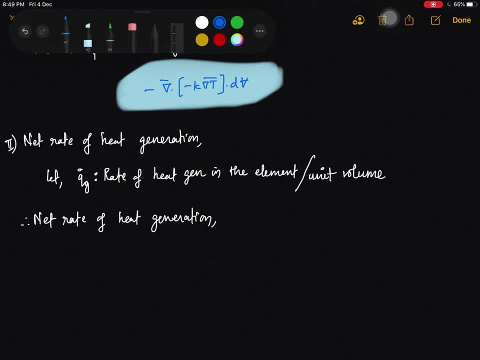 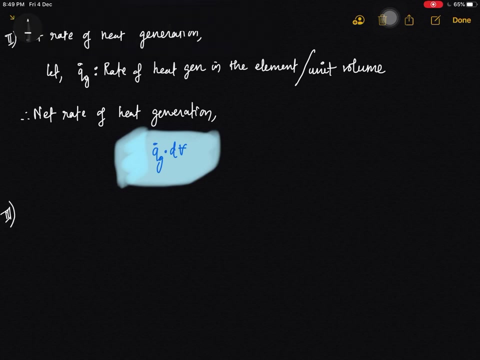 generation can be written, as can be written as 2.g, into dv, dv, dv, dv, dv, where d, v is the volume of the particular element. so this is the net rate of heat generation. okay, so next we will be dealing with third term, which is nothing but the. 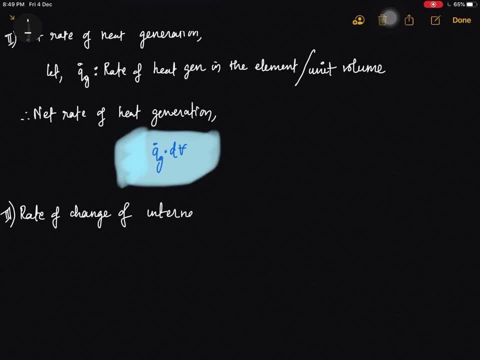 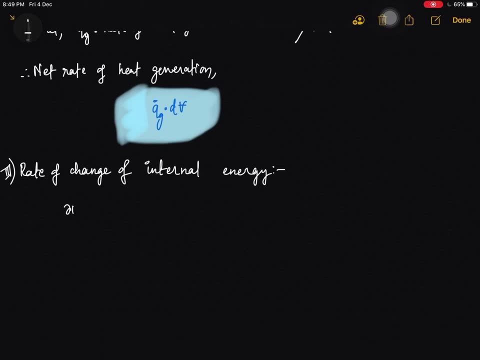 rate of change of internal energy, and this willshere written as 20.00: 20.00. dou u by dou t. where u is the internal energy, and this can be written as dou by dou t of u will be dm into c into t, okay- where this dm is the mass of differential, element of differential. 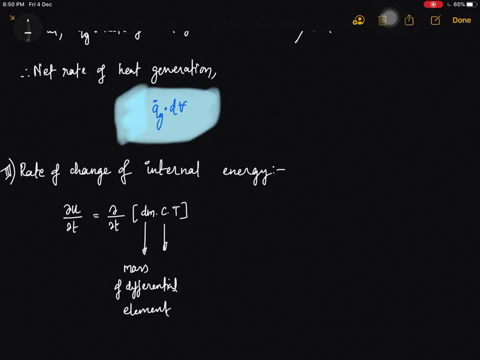 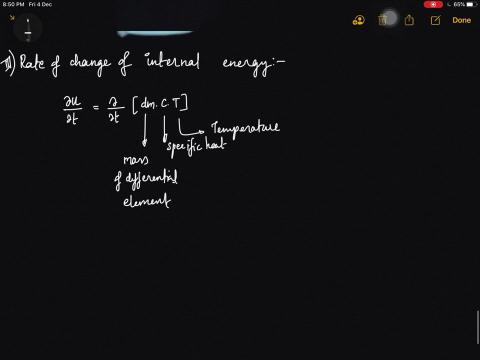 element, and this c is the specific heat and this t is the temperature. so we can write this dou u by dou t, as dou by dou t of rho into dv, into c, into sorry t, where rho is the density and this dv is the volume of the element that we considered and c. 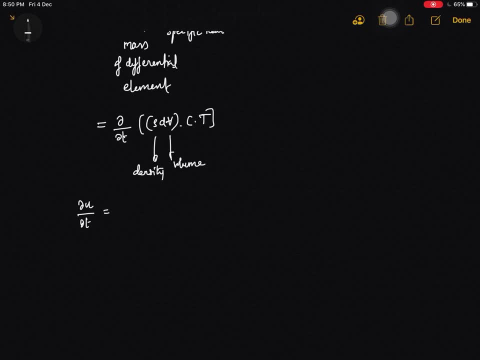 and t are the specific heat and temperature, so this can be written as dou u by dou t, which is the rate of change of internal energy, will be equal to, and this u is the capital u. please note that will be equal to rho into c, into dv, into dou t by dou t, so so rate of change of internal energy. 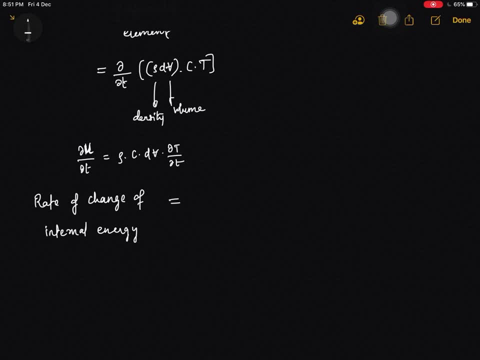 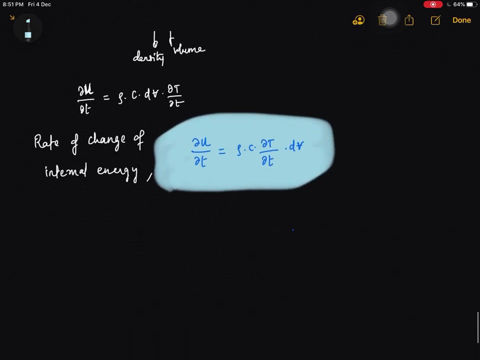 will be equal to or can be written as: internal energy can be written as: dou u by dou t will be equal to: rho into c, into dou t by dou t into dv. so this is the rate of change of internal energy system. so let's club all these three terms into one equation as: 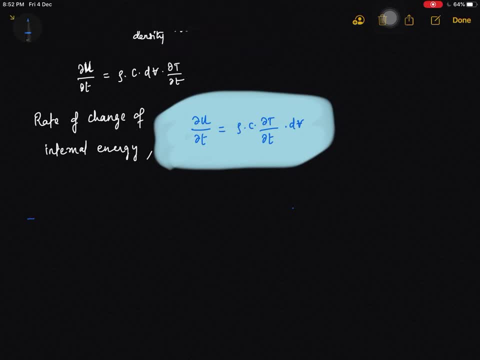 first term, which is minus del dot, minus k, delta t into dv plus into dv plus second time, that is q dot g into dv, which is a rate, a rate of net rate of a heat generation will be equal to this term, that is, rho c, d, t, b, dou t dv. 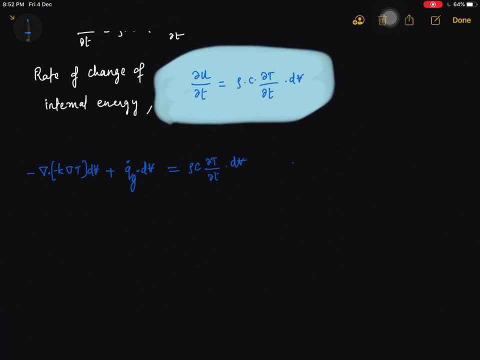 we can say dv in all these terms, so let's cancel the dv and we can write del dot k, delta T k. delta T k plus q dot g will be equal to rho c into dou t by dou t, And this is the general heat conduction equation. 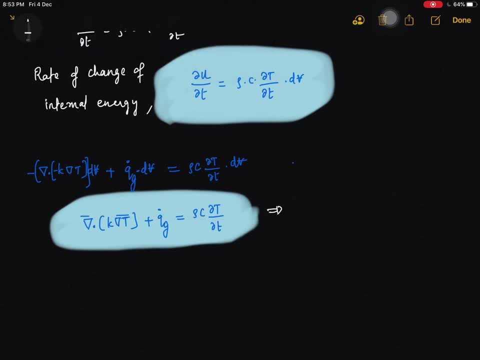 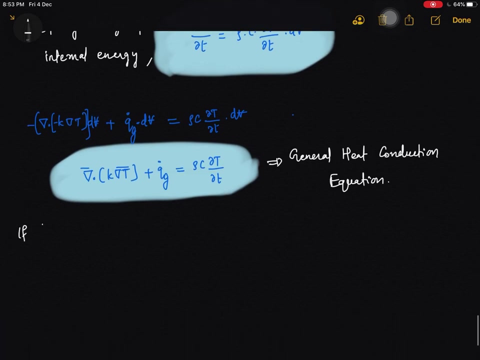 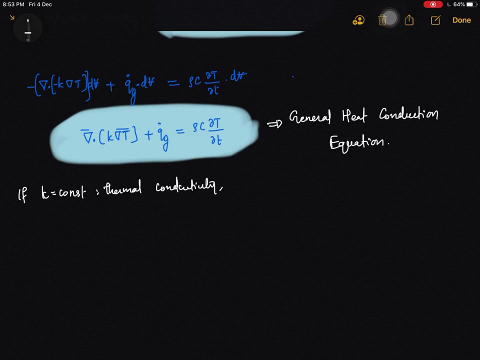 So, please note, this is the general, most general form of heat conduction equation. Okay, so suppose if k is constant, which is thermal conductivity, Suppose a thermal conductivity is constant For a particular material. for all the engineering materials we will be considering, thermal conductivity will be constant. 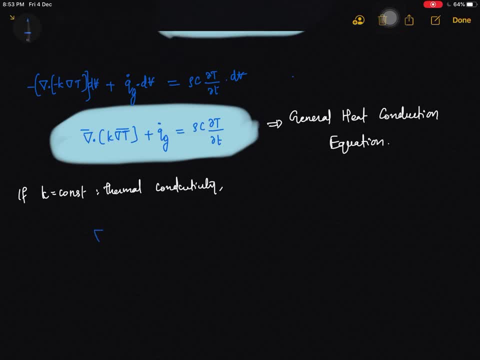 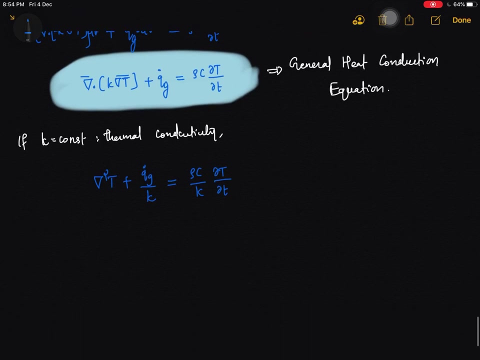 So we can write this equation as del square T plus q dot g by k will be equal to rho c by k into dou t by dou t. So this equation can be further written as del square T will be plus q dot g by k equal to 1 by alpha dou t by dou t. 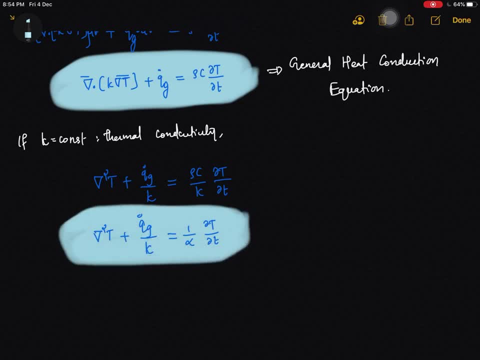 Okay, so this particular equation is called the Fourier Biot equation. This equation is called the Fourier Biot equation Where this alpha is equal to thermal diffusivity and this will be equal to k by rho c, where k is the thermal conductivity and this rho, which is a transport property, and this rho and c are the thermophysical property of the medium. 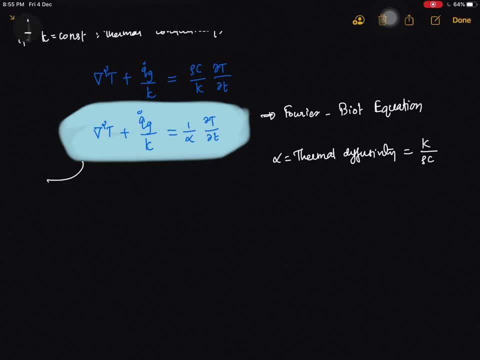 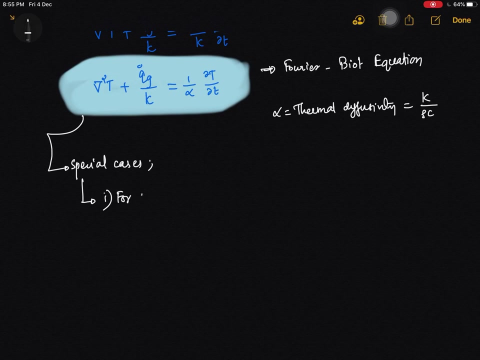 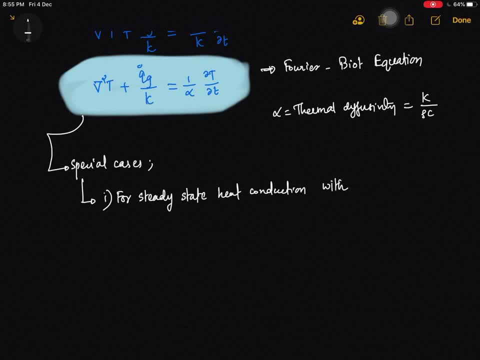 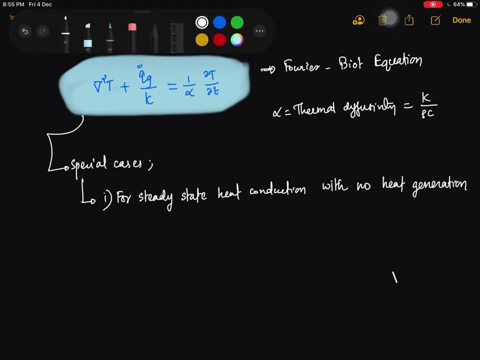 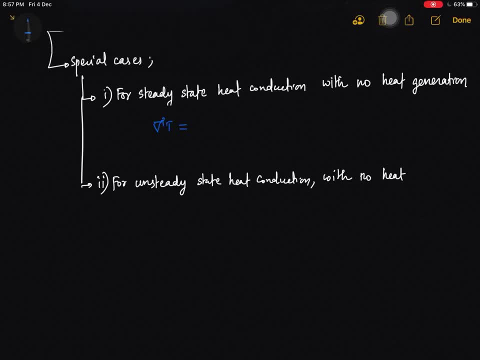 So this Fourier Biot equation will be having some special cases. be written as: del square t will be equal to. sorry, there is some error in this equation and this is having some. so this Fourier biotic equation is having. this Fourier biotic equation is: 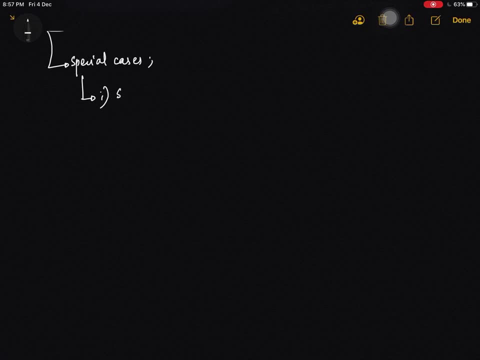 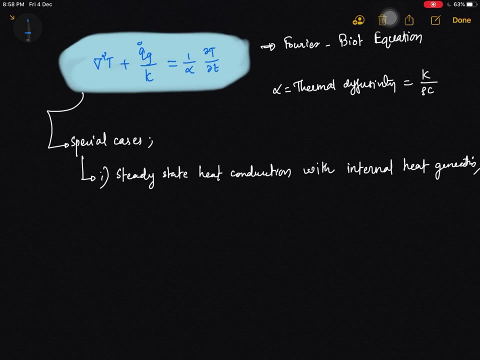 so the first special case is steady state heat conduction, steady state heat conduction with heat, with internal heat generation, with internal heat generation, with internal heat generation, and so this equation can be written as: so the first equation, that is, this del square t, this Fourier biotic equation, can be: 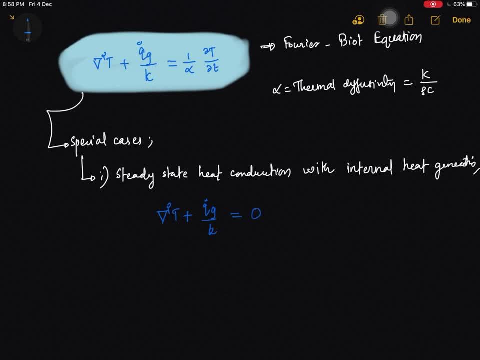 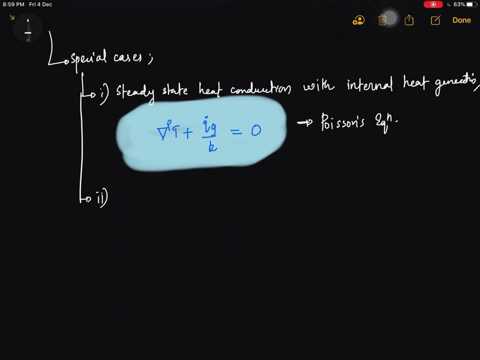 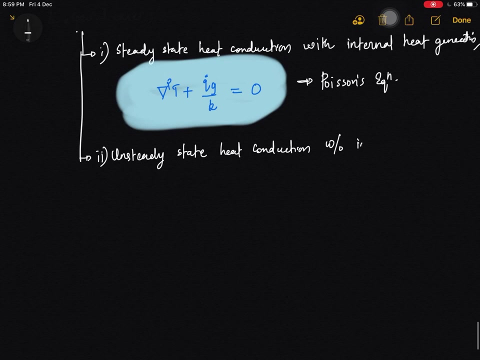 written as del square t plus q dot g by k will be equal to zero, and this equation is called the Poisson equation. and this equation is called the Poisson equation, okay, so the next special case is unsteady state. unsteady state: heat conduction without. 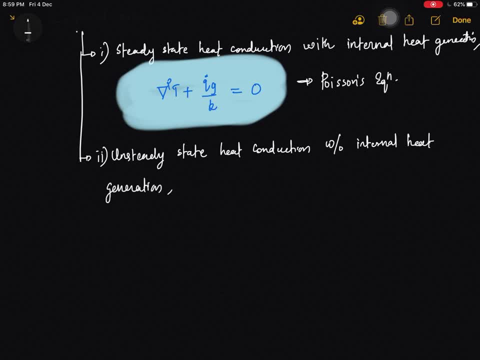 internal heat generation, and so this equation can be written as: so the Fourier biotic equation will be changed into del square t will be: is equal to 1 by alpha dot, t by 2 t. so this equation is called the famous diffusion equation. this equation is called the 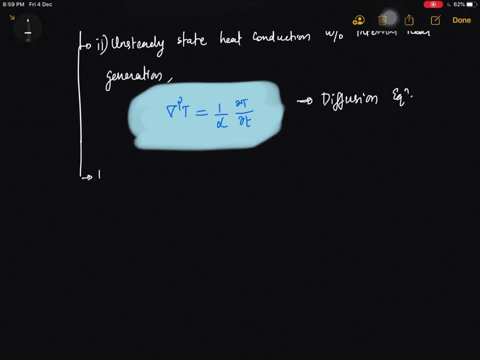 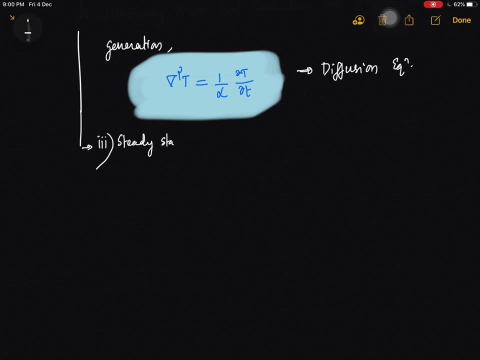 diffusion equation. so the third special case of Fourier biotic equation is: and no internal heat generation, no internal heat generation, but follow the previous vinegar encouraged الا we can write the Fourier biotic equation as del square T will be equal to 0 and this equation is the. this equation is called the Laplace equation. okay, so these are. 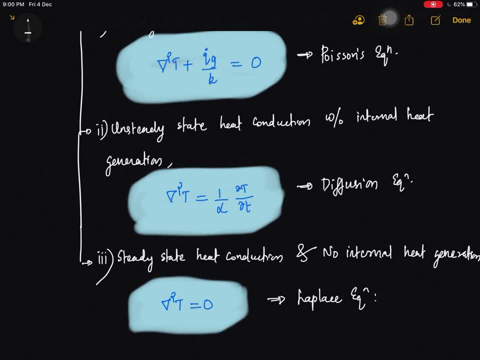 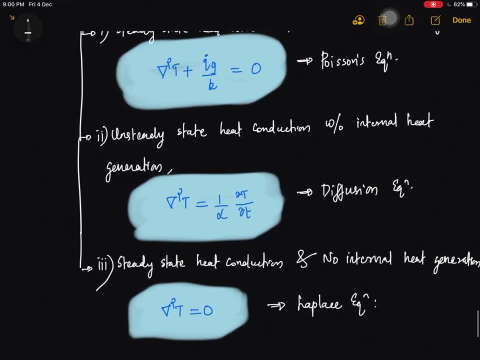 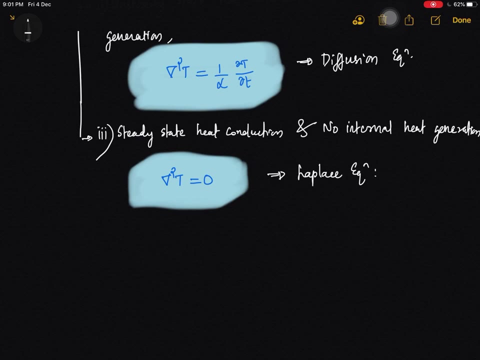 the three special cases for this particular Fourier biotic equation. these are the three special cases for this particular Fourier biotic equation, and so we can see in all these equations one del square and this del square can be converted into various coordinate systems depending upon the problems. so 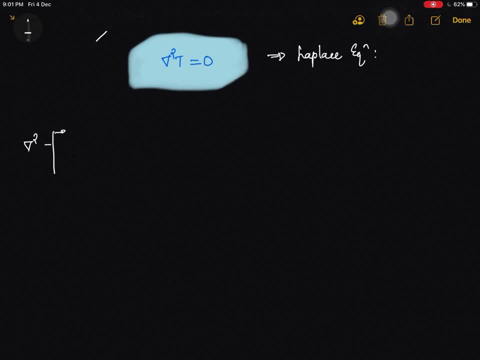 let's discuss this del square in various forms. this del square in Cartesian coordinate system. Cartesian coordinate system, we can write: del square will be equal to dou square by dou y square plus dou square by dou y square plus dou square by dou y z square. and this in the cylindrical coordinate system we can: 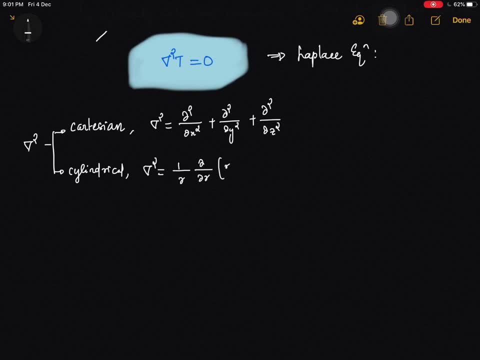 write del square, we'll be equal to 1 by R, dou by dou r, R into two by dou plus 1 by r, dou by dou phi into R, into dou by dou phi plus dou square by dou z square, and in the spherical coordinate system we can write del square will be equal to 1 by R square. 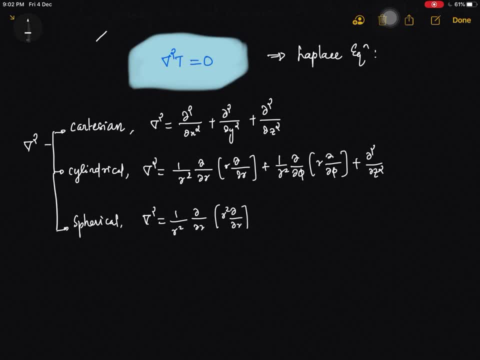 del square, so r square dou by dou r into r square. dou by dou r plus 1 by r square. dou by 1 by r square, sine square theta into 1 by r square, sine square theta into dou square by dou 5 square.